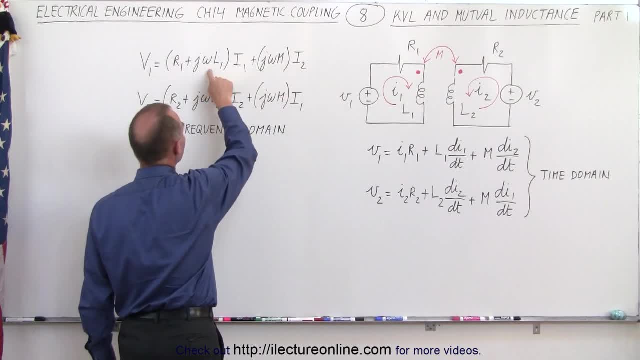 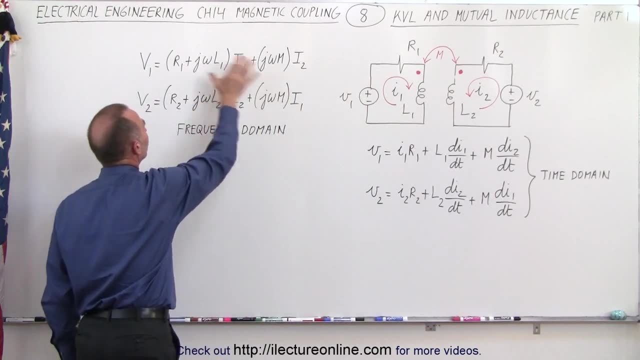 in the other circuit. So there we're going to have a j omega M instead of a j omega L. So it's going to be j omega times, mutual inductance times, the current in the other circuit which is going to add to the voltage drop in this circuit right here, And the same for the second circuit in. 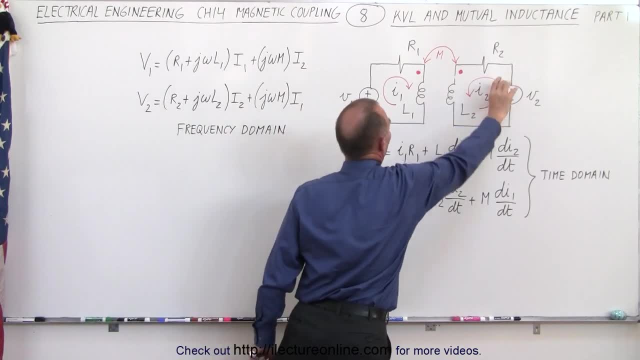 the frequency domain. Notice that the voltage drop across the, across the voltage supply, is going to be equal to the voltage drops across the resistor and the inductor, but also caused by the mutual inductance by the other circuit. So it's j omega M times the current in the first circuit which 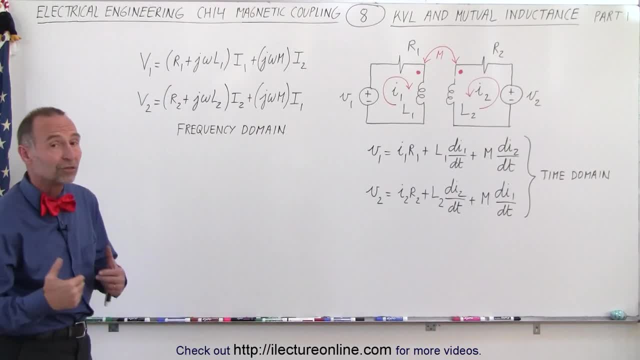 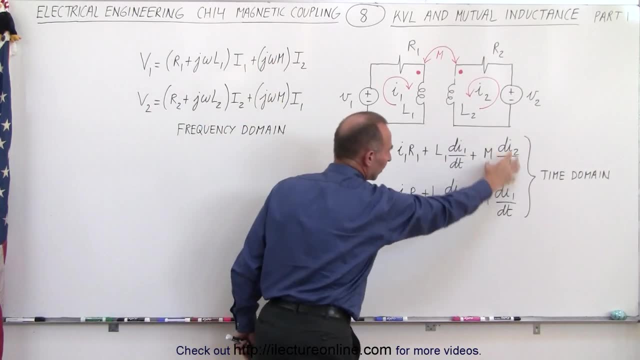 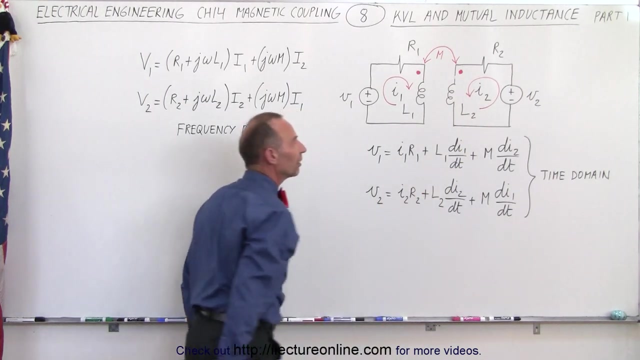 will also be affecting the second circuit. So you can see that if you use KVL on mutually coupled circuits you have to include the term that's caused by the mutual inductance. We add the term if the coupling is the same. We subtract the term when the coupling is on the opposite side of the. inductor, And that is how it's done. 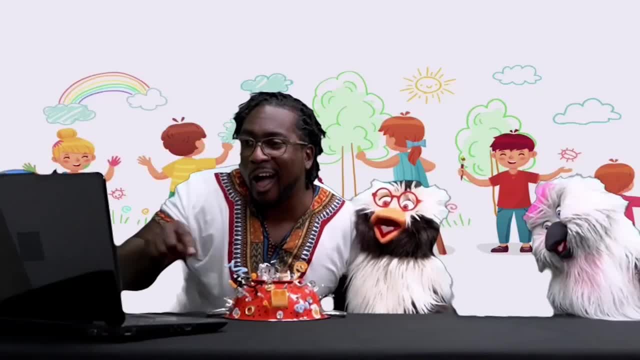 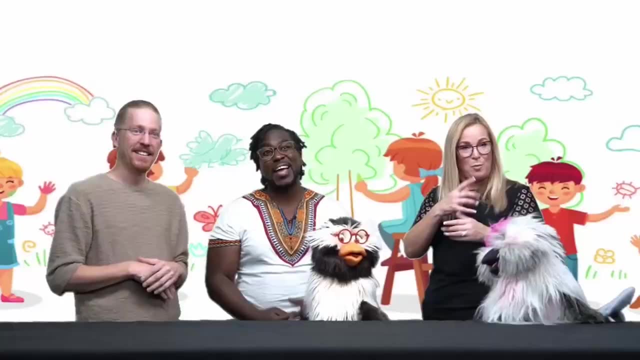 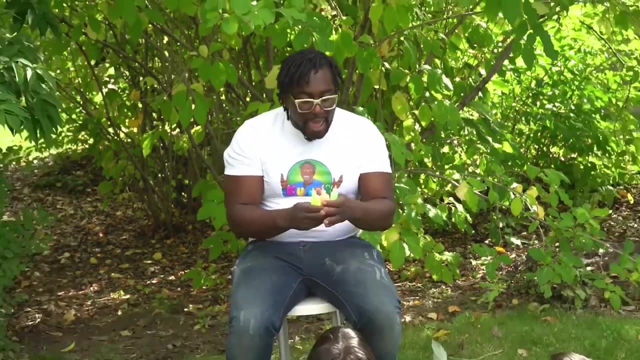 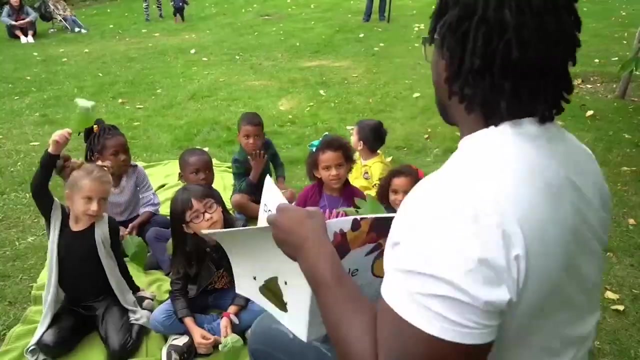 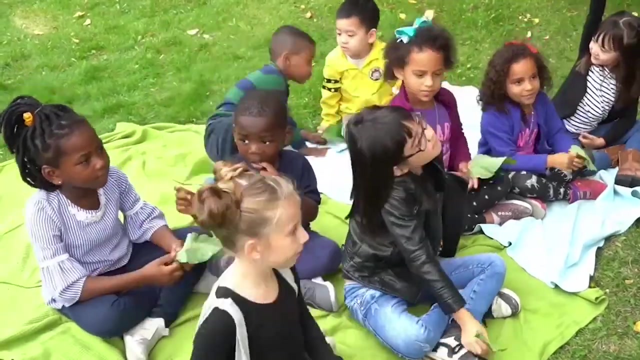 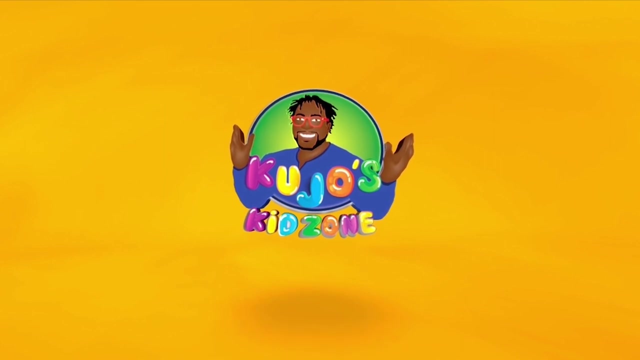 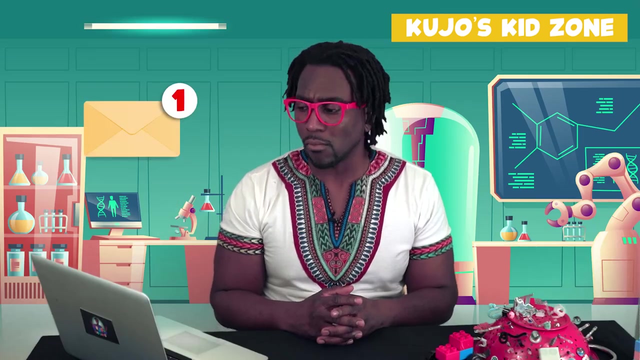 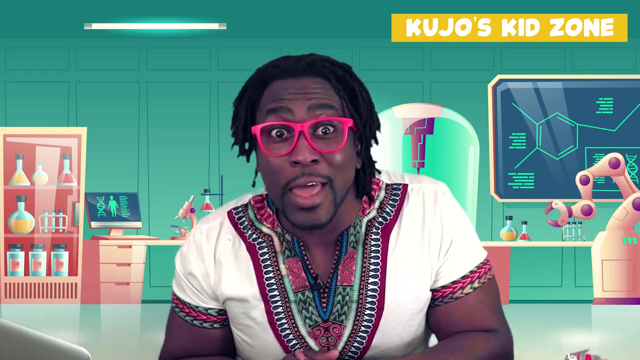 Thank you for watching Kujo Kujo. Just like you, I'm gonna be me: Kujo Kujo Kujo. Well, hello friends, So glad that you can join us today. It looks like we have a message from one of our special viewers on the computer. Let's see who it is. 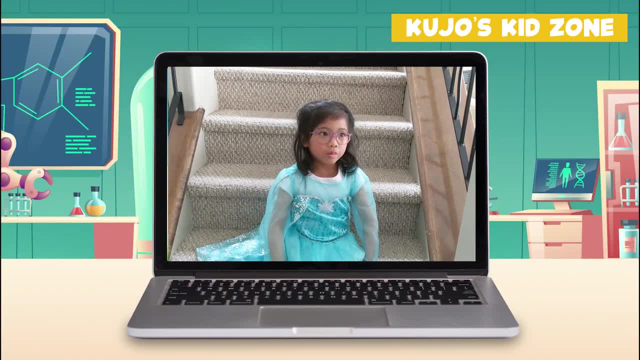 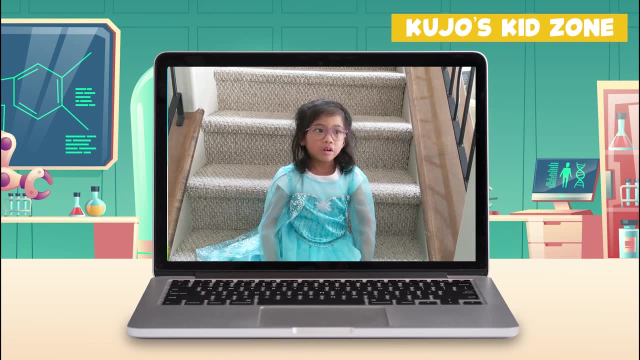 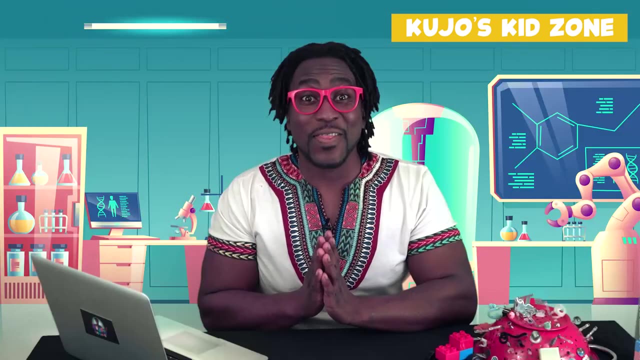 Hi, Hi Kujo, My name is Michaela And I'm five years old And I'm from Canada, And can you show me a magic trick? Thank you so much for your question. Let's try to figure this out together.